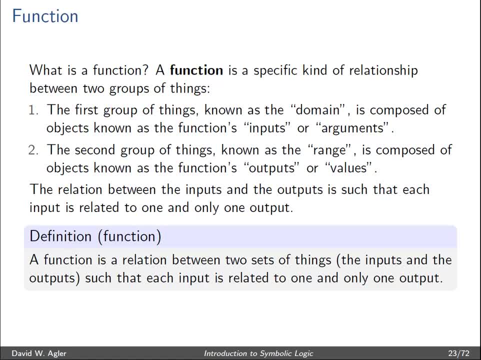 The relationship of the inputs to the outputs is such that each input is related to one and only one output. So the notion of a function is just a type of relationship between two sets or collections of things- the inputs and the outputs- such that each one is related to one and only one output. 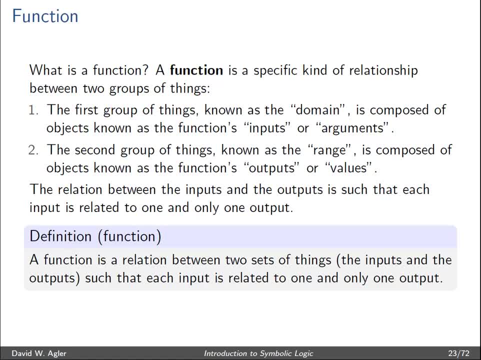 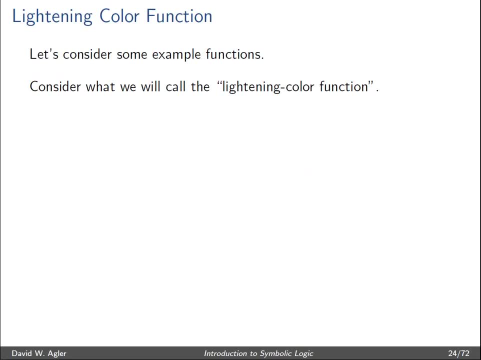 each input is related to one and only one output. So let's look at some examples to get a clear sense of what a function is. So let's consider a function called the lightening color function. This function says that take any color as an input will relate it to an output which is simply a. 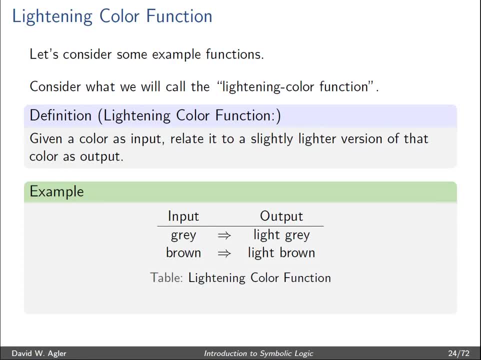 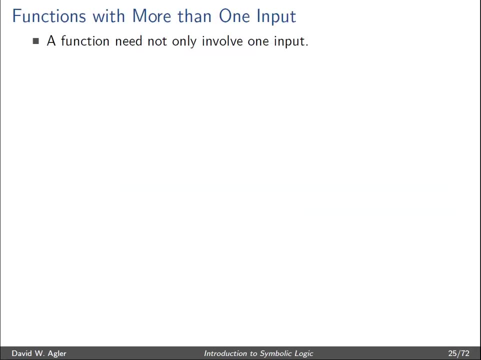 lighter version of that color. So we can think of, let's say we had a color gray as input, the output would be light gray or a lighter version of gray. If we had brown as the input or argument of that function, the output would be light brown. One thing to keep in mind is a function need not. 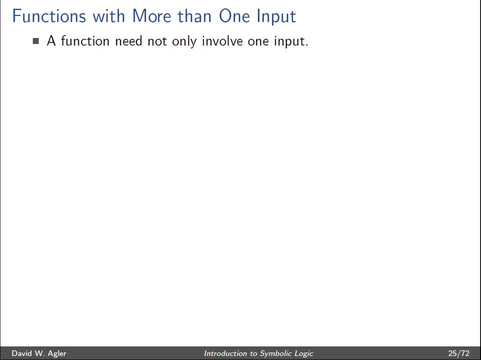 only have one input. we can have a set or group of inputs, but what's important is that set or collection of inputs is related to one and only one output. Just to repeat this point: a function can have two or three or any number of inputs, but this set or collection can. 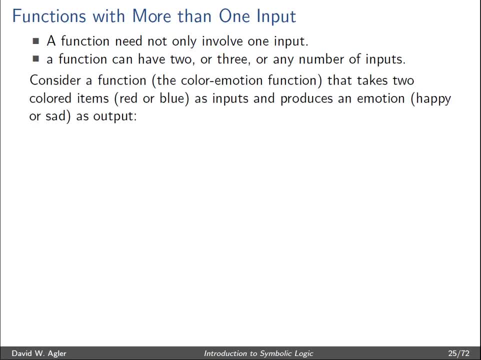 only have one input. So if we had a color gray as an input, the output would be light gray or a only be related to one and only one output. So let's consider an example and let's call this the color emotion function that takes two colored items you can imagine, let's say, pieces of clothing. 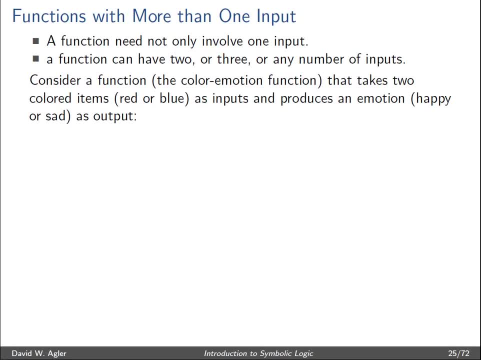 and these colors are the inputs and it relates it to one and only one output. Let's say it's an emotion and just to kind of keep the emotions, the number of emotions, constrained, let's just say it relates it to either happy or sad. Let's define this color emotion function a little bit more. 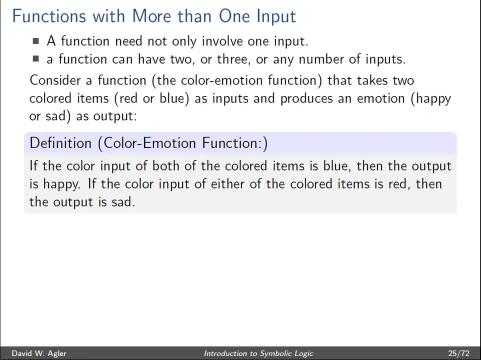 specifically And just take the domain of items as blue and red and the output emotions as happy or sad, And so the cut this color emotion function will say: if the color input of both of the color items from the domain is blue, then the output emotion will be happy. If the color input of either of the 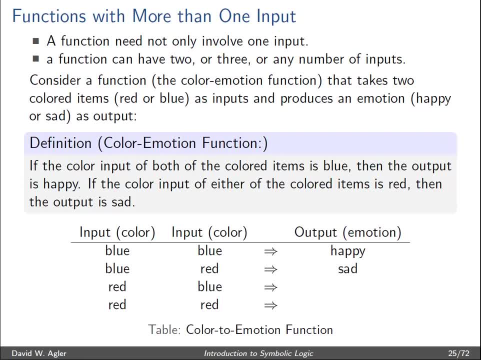 colored items is red, then the output emotion will be sad. So here's a couple example and I've kind of filled in part of the function already. If we had two colored inputs in- they're both blue, then the output would be happy. If we have one kind of color input which is blue and the other that, 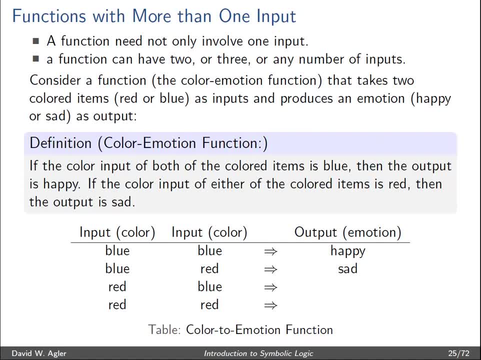 is red, then the output is sad. In addition, if we have a two color inputs, one's red and what's blew caught recordings of this color emotion function, then the output will also be sad. And if there are to read: We said that their color emotion function says that if either of the color items is read in: 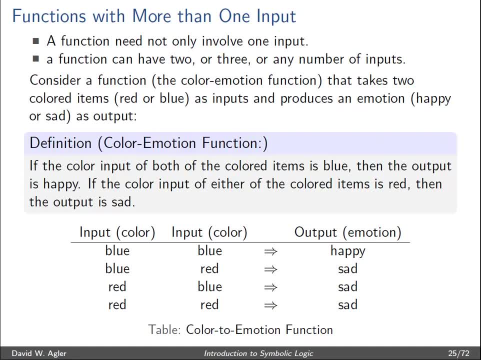 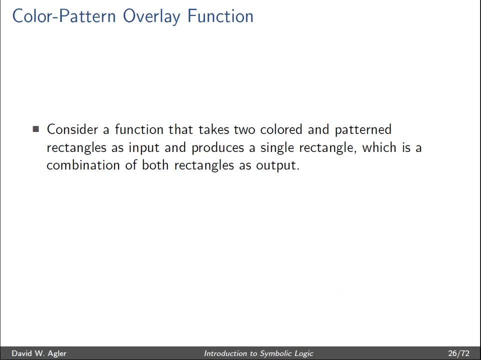 the output is sad, so the output emotion, here again, will also be sad. so let's look at one more general example of a function before we talk about functions in the language of symbolic logic. so let's take a function that takes two colored and pattern rectangles as input. it'll take any kind of combination of colored and. 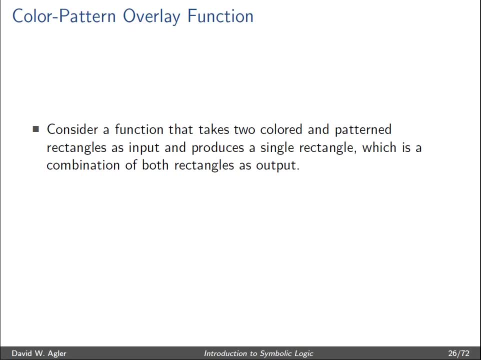 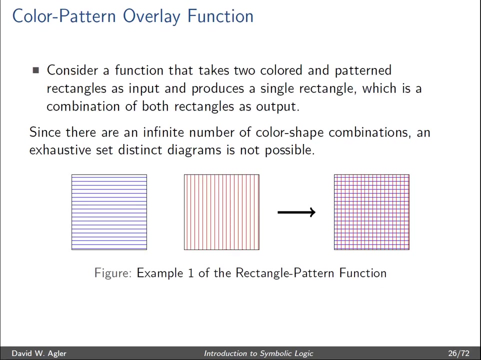 pattern rectangles as input, two of them, and produce a single rectangle as output, and this output will simply just be the overlay of the two inputs, since there are a number of. if we let the domain be any kind of possible colored and pattern, there'll be an infinite. so we'll just focus on some specific ones here. so 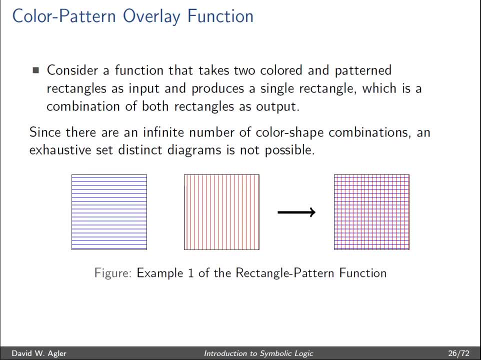 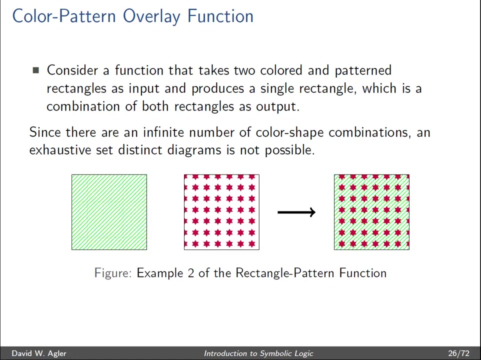 here's an example. we have two colored pattern rectangles. one is a blue square, like looking figure, with horizontal lines. the other is a square with red vertical lines and the. so those are the inputs and the output is the sort of taking those two squares and putting them on top of each other. in this second example we have again two squares as 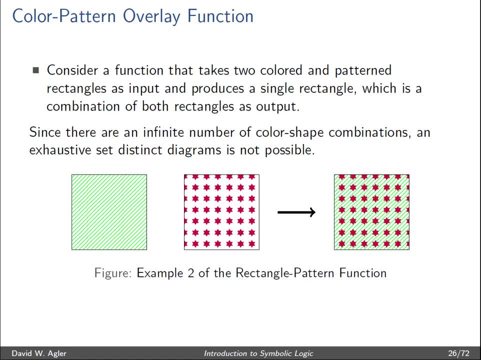 input. the first has green diagonal lines and the second has red stars. now, these two inputs, or this collection of two inputs, is related to one and only one output, and that's the overlay of the two patterns, where there is a square with red stars as well as green diagonals. so what does this have to do? 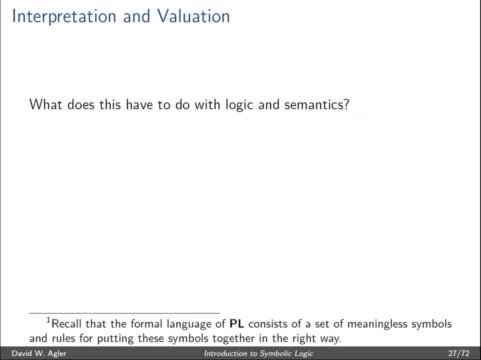 with logic and, more importantly, what does it have to do with the semantics of logic? so the semantics of the language of propositional logic involved two important functions. the first function is what's called the interpretation function. now, this function takes propositional letters, single propositional letters, as input and 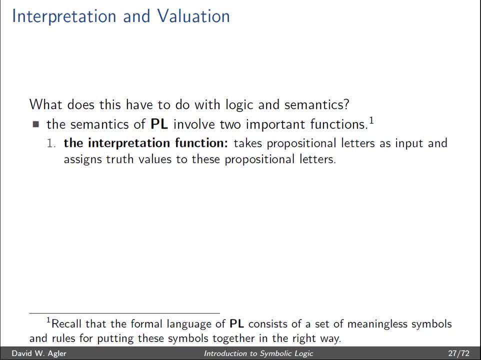 assigns truth values to these propositional letters. so it'll take a propositional letter and relate it to one and only one truth value, either true or false. but we'll talk about more talk. more about this in a second. the second function is known as the evaluation function and this assigns a truth value. 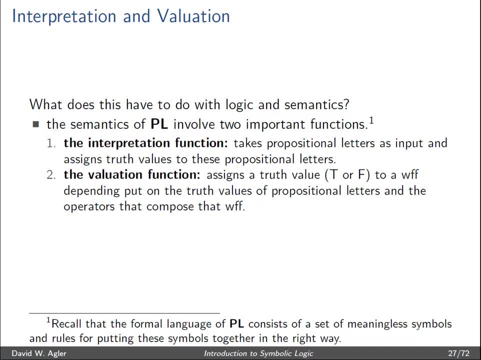 to a well-formed formula, depending upon the truth value of the propositional letters and operators that compose that well-formed formula. so, essentially, this one takes the truth value of components of a formula and relates it to one and only one truth value as an output. so let's 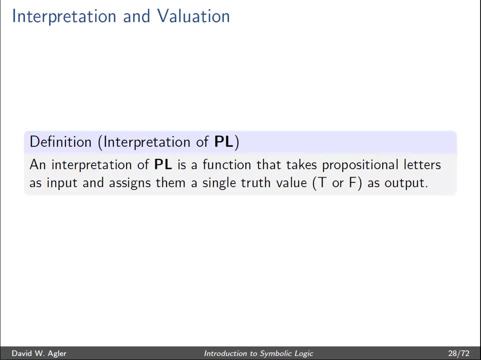 look at each of these now. the interpretation function is a function that takes propositional letters as input and assigns them a single truth value, true or false, and we'll breathe that. abbreviate this as T or F as output. to symbolize this interpretation, we'll call it the trough that Judd and 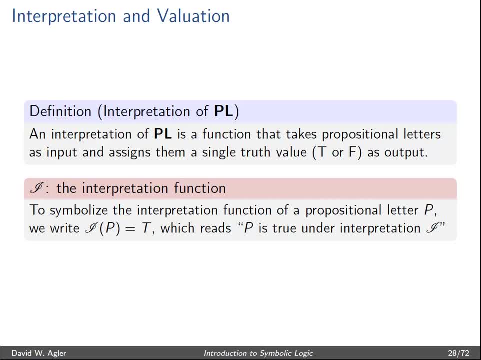 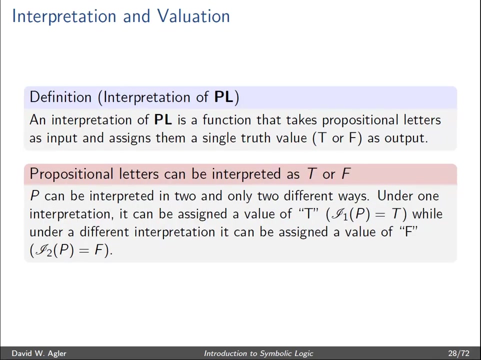 function. we could simply write I: P equals T. This is to say that the interpretation of the argument or input P has a value or output of T, which is true. Another way to read this is P, the propositional letter. P is true under the interpretation. I. Now propositional letters can: 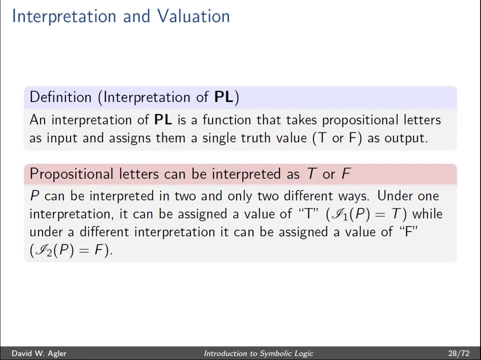 be interpreted in one of two ways. A can be interpreted as a single propositional letter can be interpreted as true and under a different interpretation it can be interpreted as false. So if we had a different interpretation, let's say it's I sub 2, then P could potentially be. 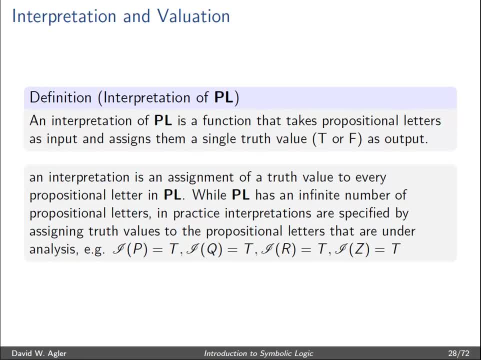 false under this interpretation. Now it's important to realize that an interpretation is an assignment of truth values to every propositional letter that is under analysis. Now there might be an infinite number of propositional letters in our language, but just when we go to analyze an argument or look at a set of formulas and kind of assess that we can just 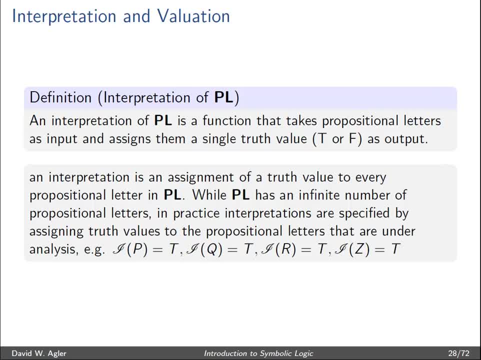 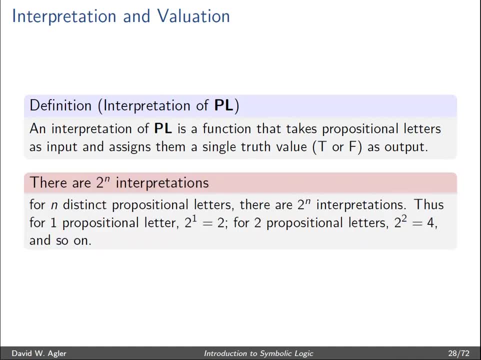 simply indicate the interpretation of each propositional letter we're interested in by simply writing I P equals true, or I Q equals true, and so forth and so on. So one question we may ask ourselves is: how many interpretations are there for n distinct propositional letters? 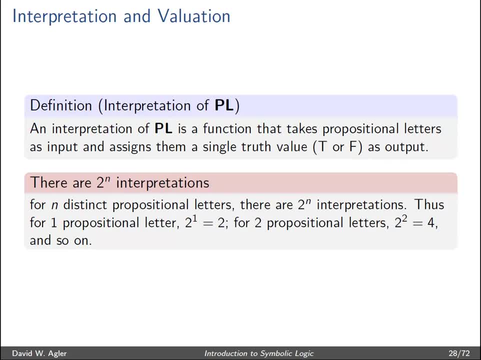 That is, if I'm looking at an argument or a formula. how many different ways can I assign truth and falsity to the propositional letters found in that formula? Well, the answer to that is determined by the formula 2 to the n, where n is the distinct. 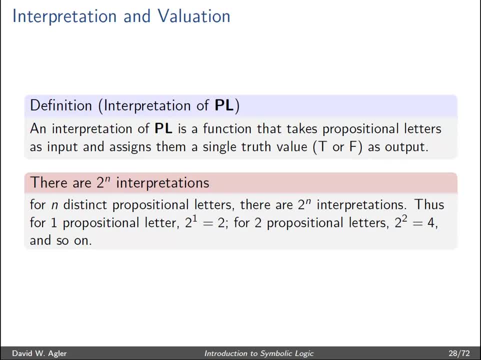 number of propositional letters. So, for example, if there's one propositional letter, let's say it's P, there's two ways to interpret it. We can interpret P as true or we can interpret P as false. For two, 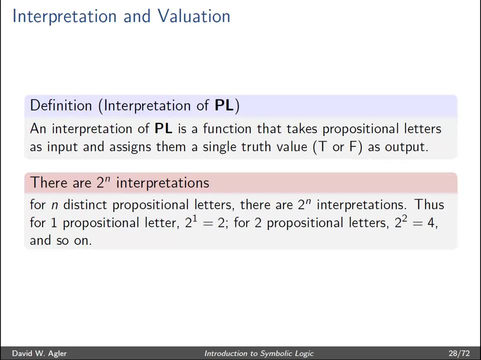 propositional letters. let's say P and Q. there's 2 to the 2 interpretations, that is four interpretations. That is, we can interpret P and Q as true. we can interpret P as true and Q as false. we can interpret P as false and Q as true, or we can interpret: 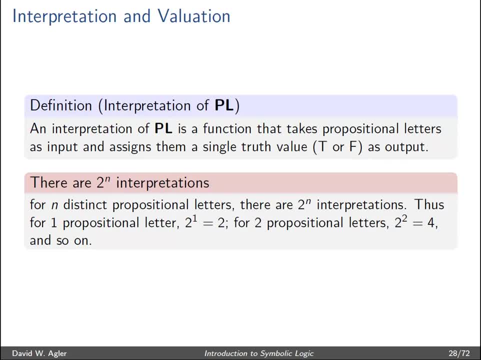 both P and Q as false. We'll talk a little bit more about that in the next class. We'll talk a little bit more about this later, but I just wanted to point this out- that we can use this formula to determine how many. 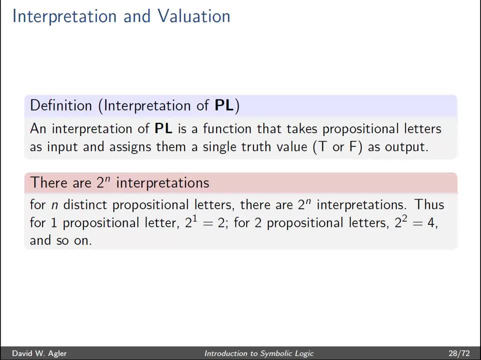 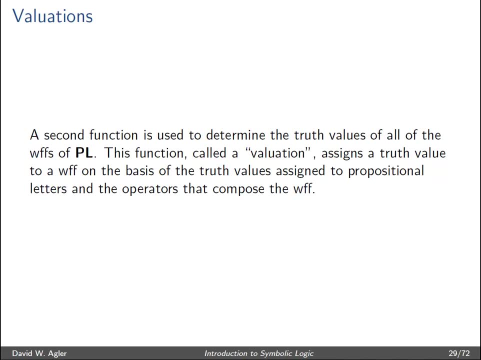 interpretations are required to give an exhaustive set of interpretations. Now I want to talk a little bit about the second important function involved in propositional logic semantics. If the interpretation function is used to determine the truth values of the different propositional letters, the valuation function assigns a truth value to. 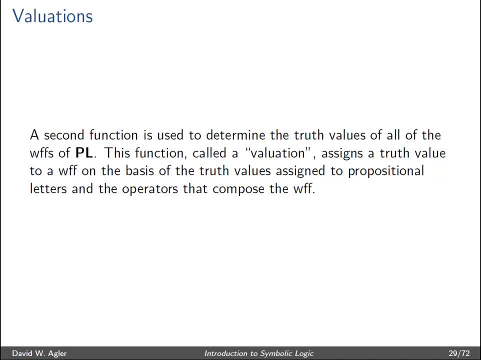 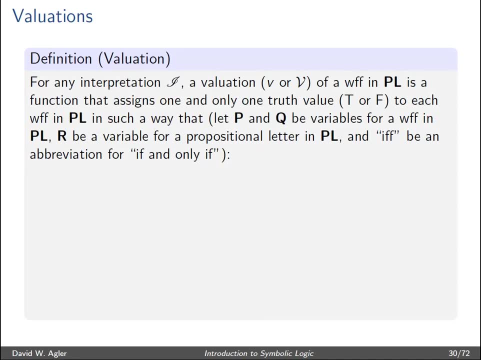 well-formed formulas on the basis of the truth values assigned to the propositional letters and operators that are found in this well-formed formula. So let's look at how this is done. So for any interpretation, and we'll just say that this is I. 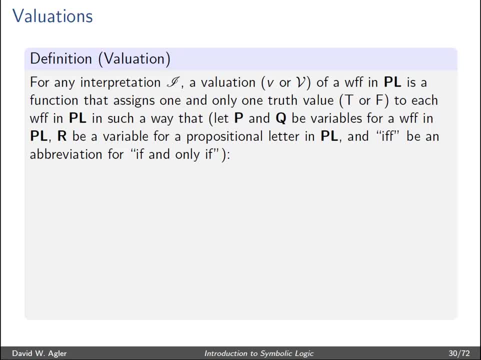 we can define a valuation function of a well-formed formula in the language of propositional logic, and this is a function that assigns one and only one truth value to each well-formed formula in such a way. So let's look at some examples Now. if r is interpreted in a particular way, 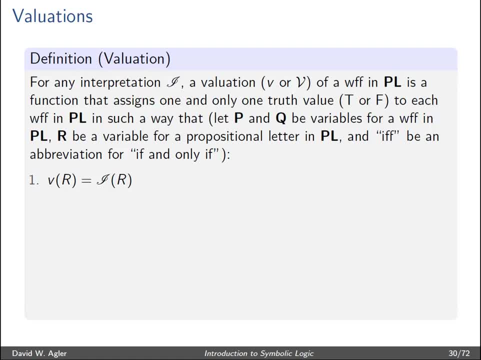 the valuation function doesn't change anything about this. It says: if r is interpreted as true, then r is evaluated as true. Recall that a single proposition is a well-formed formula and so for the valuation function of that value function, it leaves the truth value of the propositional letter alone. So if r is true, then under a particular interpretation, then the 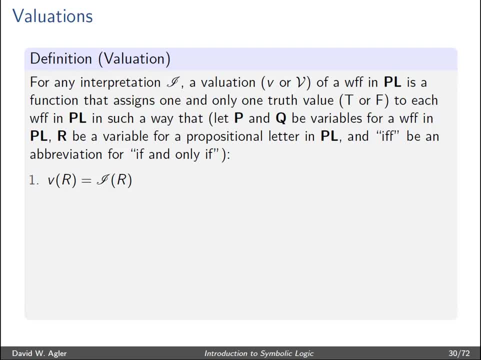 evaluation of r is going to be true. If r is false, then the evaluation also will be false. Where things get a little bit interesting is when let's say we have a formula that is a negated formula, So let's say we have not p. Now this is defined that if the 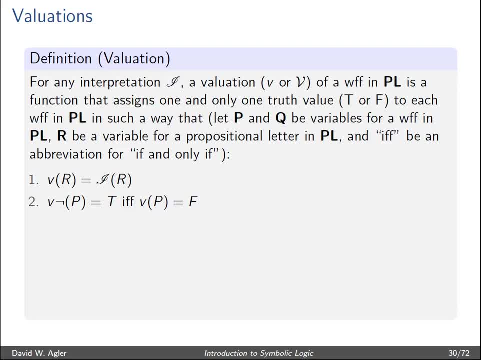 evaluation of p is false, then the evaluation of- not p, will be true. Next, how about the evaluation of p and q? Under what conditions is this the case? What's the case if the input is such that both of the conjuncts p and q are both true? That is the. 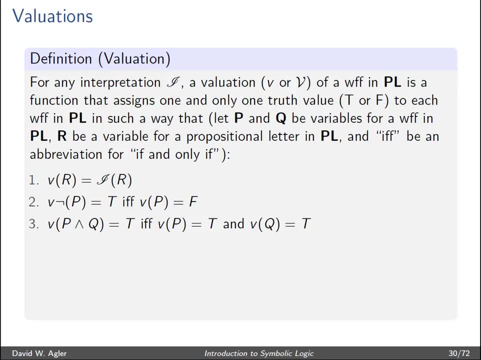 evaluation of p caret. q is true if, and only if, the evaluation of p is true and q is true. The evaluation of p or q, that is, p- vq, is true if, and only if, one or the other or both of the disjuncts are true. That is the. 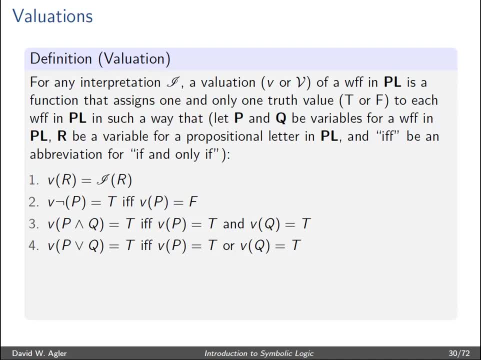 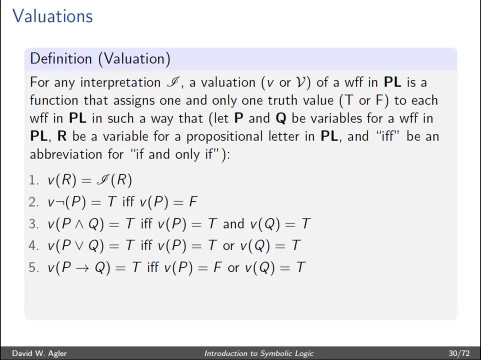 Next- and we'll talk a little bit more about this one in another video- the evaluation of p or q is true if, and only if, either p is true or q is true. where the valuation of P is false or the valuation of Q is true, then the 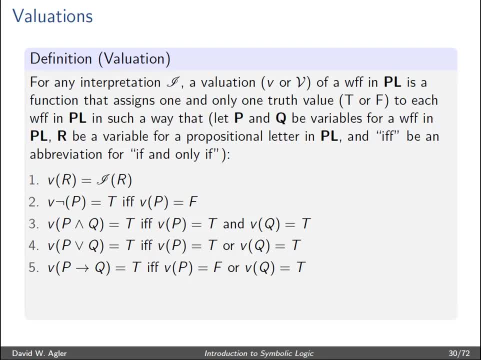 valuation of the complex, well-formed formula P- right arrow Q will also be true. finally, the valuation of P double arrow Q is true in one of in either of two cases: in the case where both P is true and Q is true, or in the case where the valuation of P is false and Q is false. so if the interpretation function, 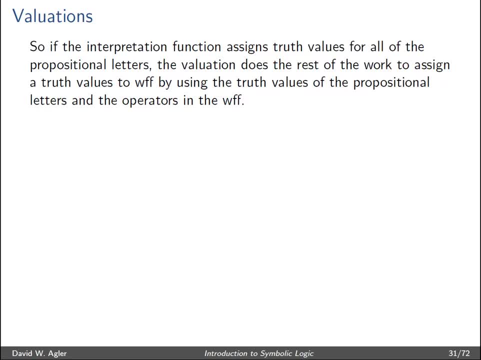 assigns truth values to all the propositional letters. the valuation function does the- what we might say- the rest of the work by taking the assignment of truth values to those propositional letters and using them with various valuation rules to assign truth values to the well-formed formulas. 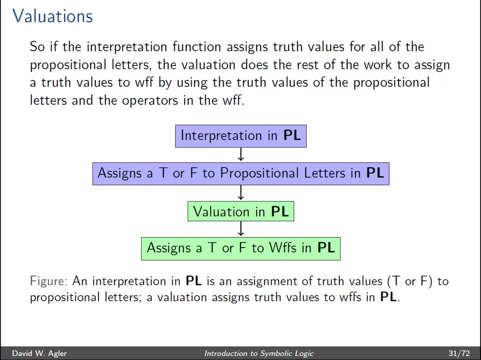 and so you can think about it using this diagram. we have an interpretation, and what does it do? it takes every single propositional letter that we're interested in and assigns it a value, true or false. then we have the valuation function, and it will take those interpretations and use them, associated with various valuation rules, to assign a. 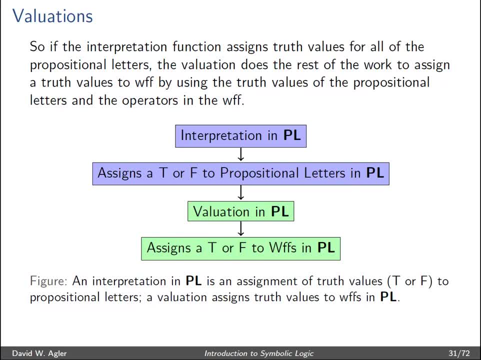 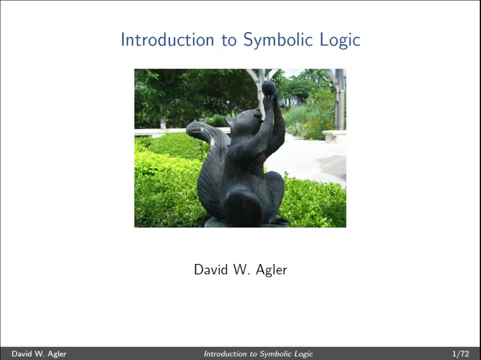 truth, value T or F to every complex, well-formed formula in the language. alright, ladies and gentlemen, this has been another video on the language of propositional logic. like the video if you thought was helpful, and subscribe if you're interested in learning more about the language of propositional logic and.